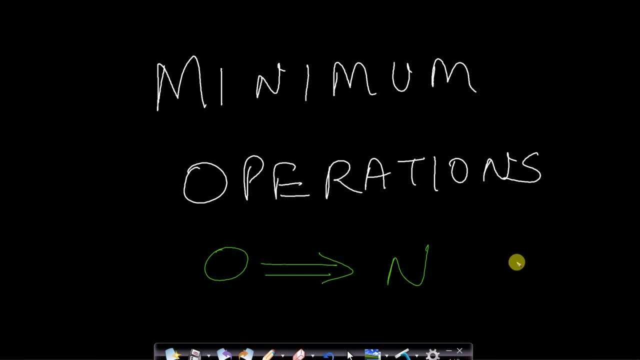 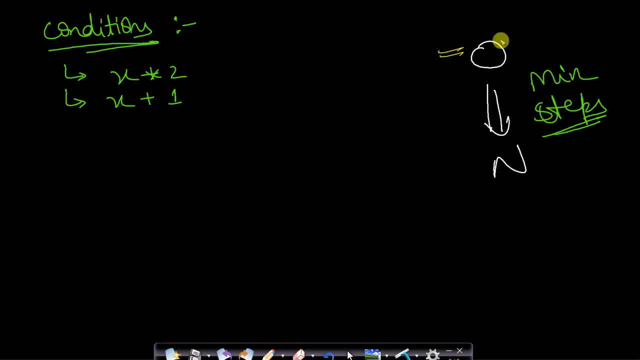 Hello guys, welcome back to take dose, and in this video we will see how to find the minimum number of operations required in order to convert 0 to n, with some given operations under some given conditions. So let us look at the problem statement. Let us say we have a number 0 and 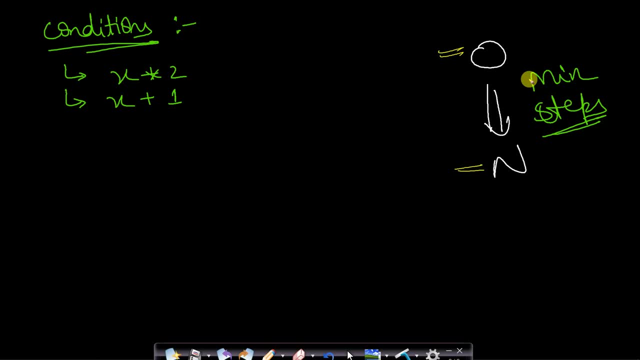 you input a number n, Then what will be the minimum number of steps in order to convert this 0 to n? and the operations allowed are given a number x at any instant, x, you can multiply it by 2, or you can add 1 to the number x and you will have to just do this conversion in minimum number of. 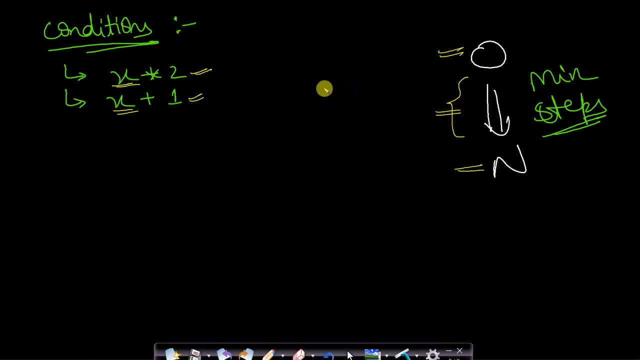 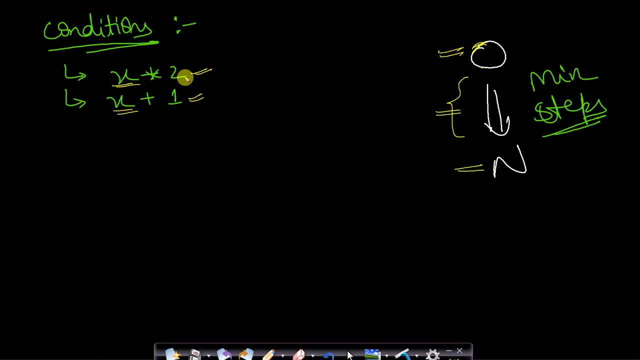 It's saying you need to convert this 0 to n and you have all these operations. Now, at any given instant, x, any value, can have 2 possible operations. Okay, either you can multiply it by 2, or you can just subtract, or you can add 1 to it. Now, if you get a value, say y, and here you get a value z, again, 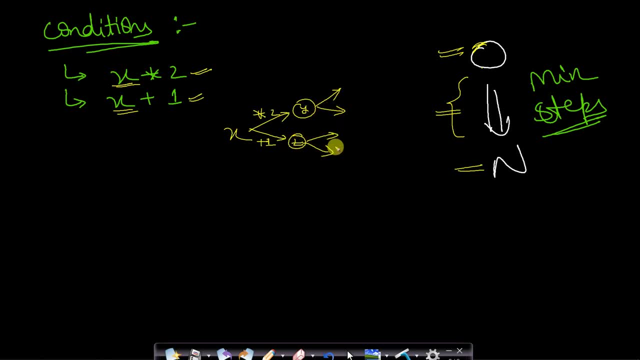 you will have 2 branches. that means 2 possible operations and like this, you will have again 2 options. Okay, so this can take exponential time if you do it by using backtracking. so this is not a feasible approach. backtracking or recursion is not a feasible approach. it will take you exponential. 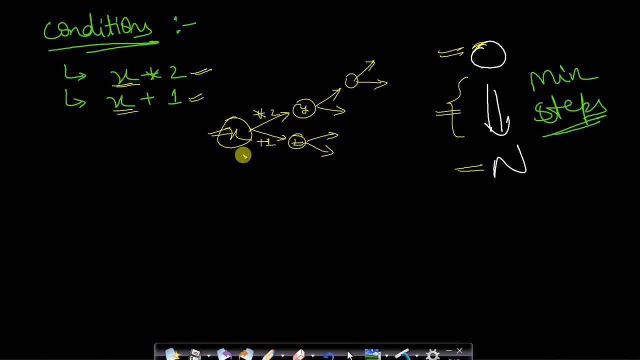 time, okay. so how to do it with a better approach? now, instead of converting this 0 to n, what i will do is i will convert this n to 0. the steps, the minimum steps to convert this n to 0 and 0 to n will always be equal. think about it. it should always be equal, okay? so if you are converting, 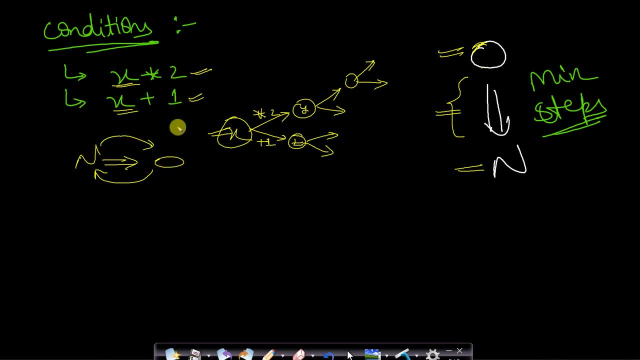 this n to 0, operations will be different. operations will be just the opposite. when you were converting this 0 to n, you had multiply and addition. so when you will convert this n to 0, you will have division and subtraction. okay, so these will be the operations, how you will swap it now. 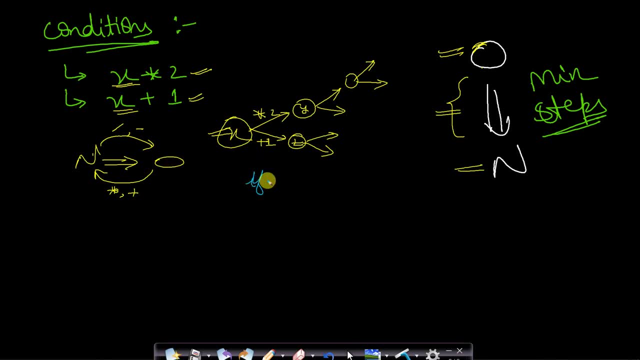 let us look at the approach. if, say, if the given number at any instant, x is, say is even, then the operation will be x equals to x by 2. else, if it's not even, then it will be odd. obviously you will do x equals to x minus 1. 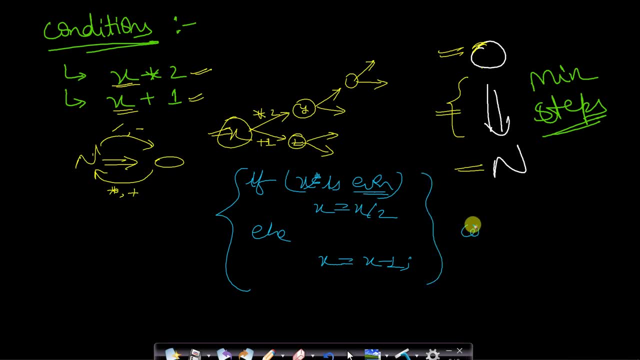 okay, and whenever you do this operation you will just increment count by 1, so count plus equals to 1. at the end you will just return the result as count. so this will be the number of operations. number of the minimum number of operations which is required. 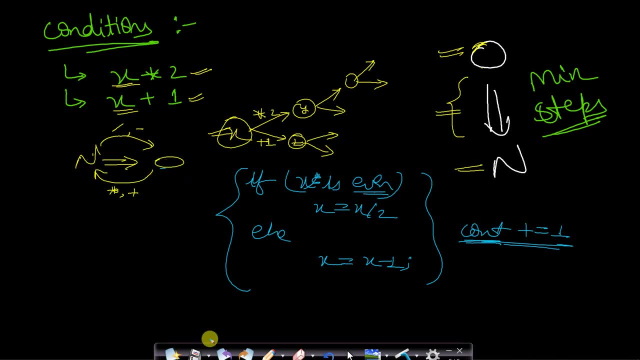 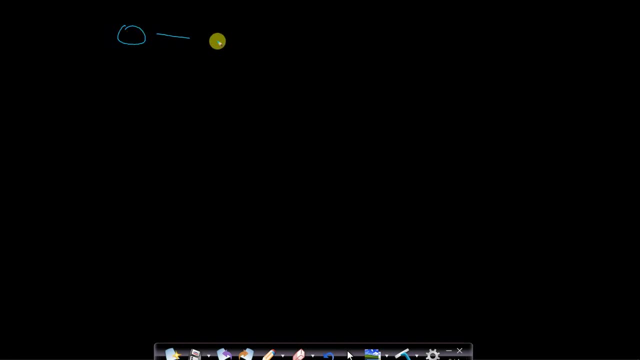 to convert 0 to n or n to 0. so let us take an example and understand it clearly. let us say you are given to convert this 0 to 12 and you are required to find the minimum number of operations. okay, so what will be the minimum number of operations? what i will do is i will take this 12. 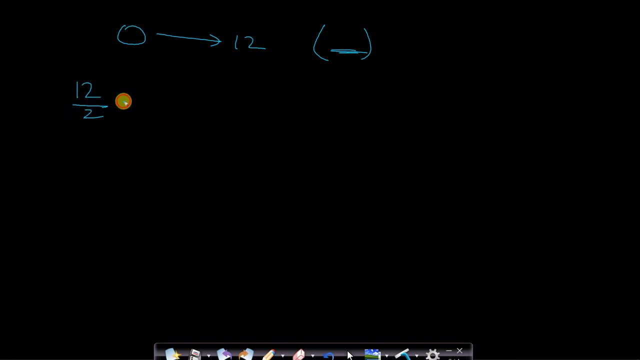 since this 12 is even, i will divide it by 2: it will be 6.. 6 is even, i will divide it by 2: it will be 3.. 3 is odd, i will subtract 1 from it. it will be 2.. 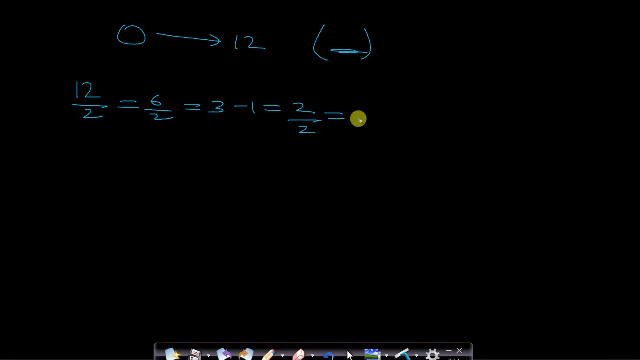 now 2 is even, i will sub. i will just divide it by 2, it will be 1.. 1 is odd. i will just subtract 1 from it and it will be 0.. now 0. we should convert n to 0. 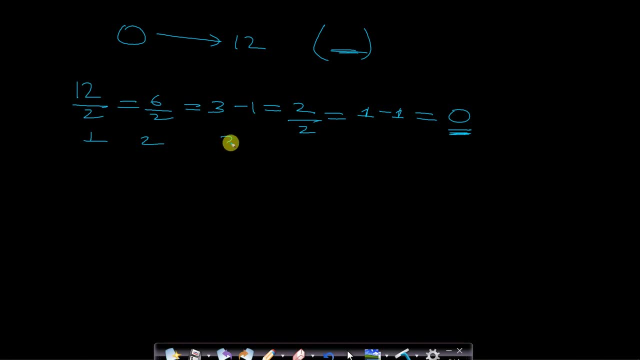 okay, so what are the number of steps? this is step 1, 2, 3, 4, 5. okay, so we are basically converting 12 to 0 in five steps steps. therefore, it should be possible to convert 0 to 12 in just 5 steps. okay, so the answer for it. 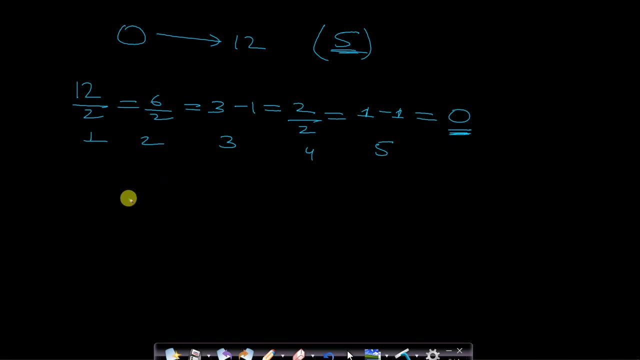 will be 5. now let us look at some another example. let's say you have a number 9. now you need to convert this 0 to 9 in minimum number of steps. now how will you do it? i will take this n value, which is 9. 9 is odd number. therefore, you will subtract 1 from it. it will be 8. 8 is even you. 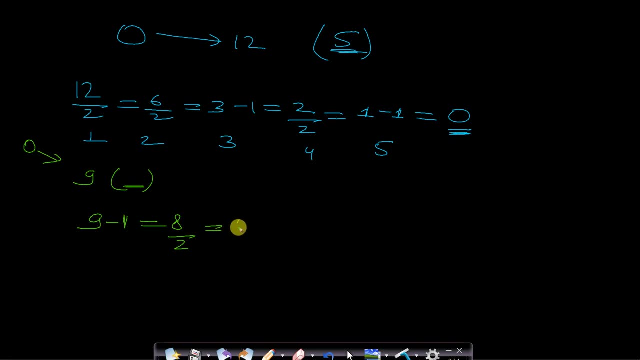 will just divide. divide it by 2, it will be 4. 4 is even. you will divide it by 2, it will be 2. 2 is even. you will divide it by 2, it will be 1. 1 is odd. you will just subtract it by 1, it will be 0.